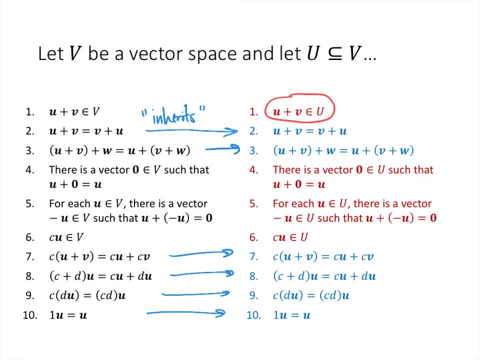 didn't add them together. we're not guaranteed that that element is still in the subset U. We're not guaranteed that the zero vector has to be in the set capital U. We're not guaranteed that when we multiply by a scalar, that that result is going to be in capital U. Now number five: here the 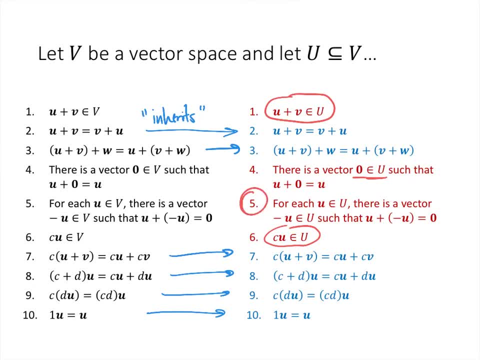 negative, the additive inverse here. if we have closure under scalar multiplication, then six is going to imply five here, because we just use the scalar negative one. and if negative one times U is in U, then that's going to imply that minus U. 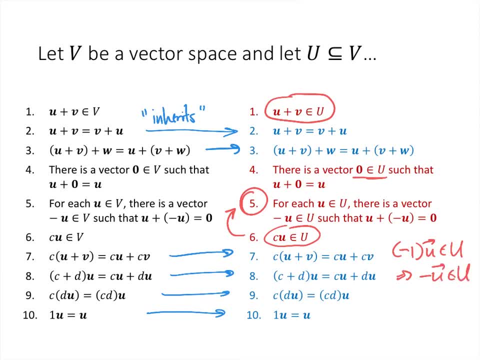 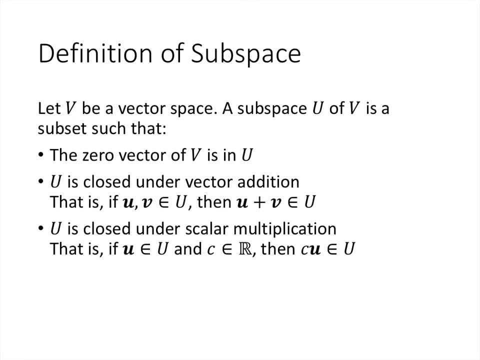 the additive inverse is going to be in U, So the ones we need to worry about are axioms one, four and six. So here's our definition. If capital V is a vector space, then a subset U is a subspace as long as the zero vector of V is in U and. 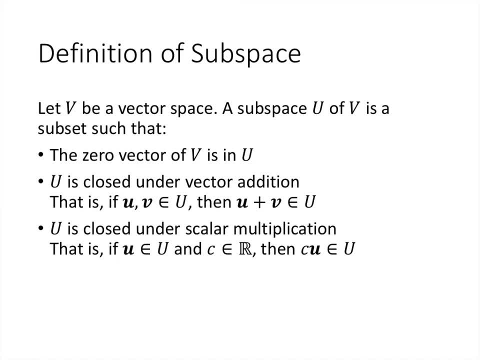 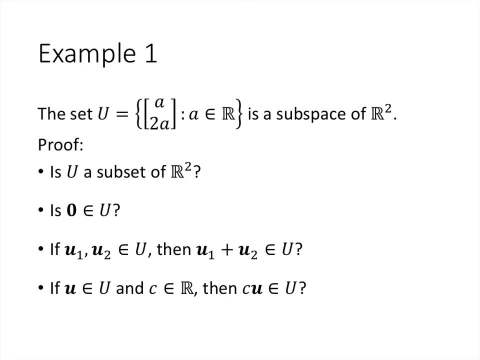 as long as U is closed under vector addition and closed under scalar multiplication. So let's go ahead and take a look at this. So let's take a look at this. So let's work through a few examples here. So if we've got a set here which is a subset, 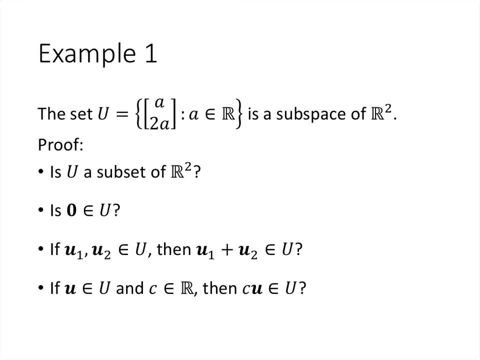 of R2, so this is vectors that look like a and then 2a as its entries, where a is a real number. is this a subspace? Well, in order for it to be a subspace, we have four things that we have to show. First of all, we have to show that it's 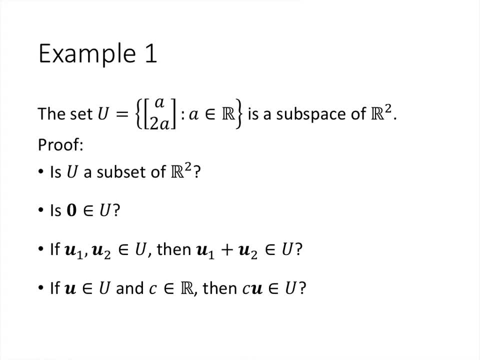 actually a subset, and then we have to show that it contains the zero vector, then we have to show that it's closed under addition and then, finally, we have to show that it's closed under scalar multiplication. So, first of all, is it a? 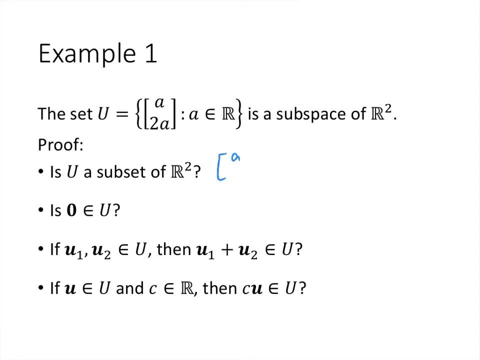 subset. Well, that's clear, right. Any vector that looks like a 2a, that is certainly an element of R2, and so that means that the set U is a subset. Is the zero vector in capital U? Well, yes, because we can let little a be 0 and the vector 0, and then 2 times 0, that. 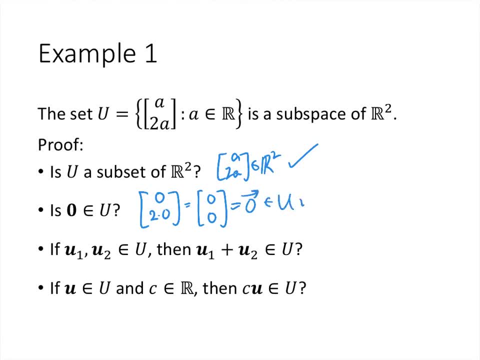 is the vector 0, 0,, which is the zero vector, and that's in capital U. If we have two of these vectors and add them together, do we get another vector in capital U? And again, the answer is going to be yes, because we can take a vector. 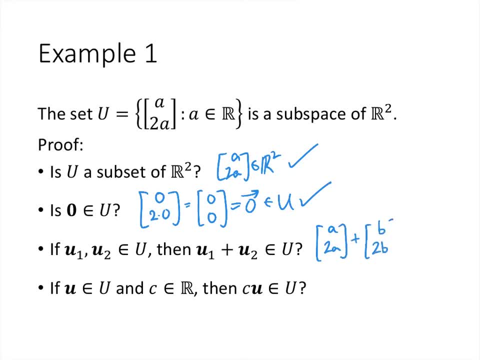 a- 2a and add it to another vector. that looks like that. maybe we'll call that b- 2b and when we add those together we get a plus b, and then this is going to be 2 times a plus b, and that's what the elements of capital U look like, and so 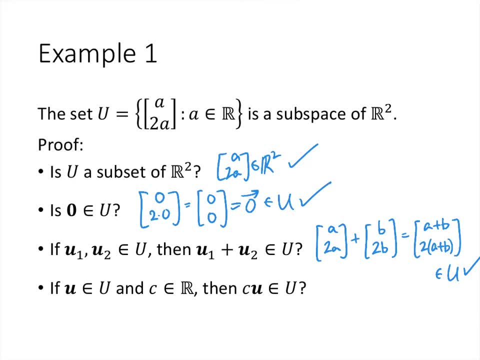 that's in capital U. Finally, if we take a vector from capital U and multiply it by a scalar, do we get another vector in capital U? And again the answer is going to be yes, because if we take c times the vector a, 2a, we're going to get the 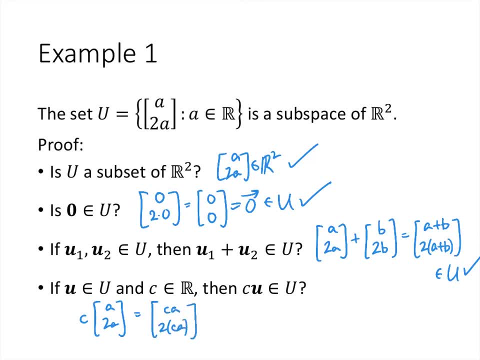 vector ca and then we can write that as 2 times ca And that's what the vectors in capital U look like. so that's in capital U. So that means that this is a subspace. Here's another example. If capital V is, 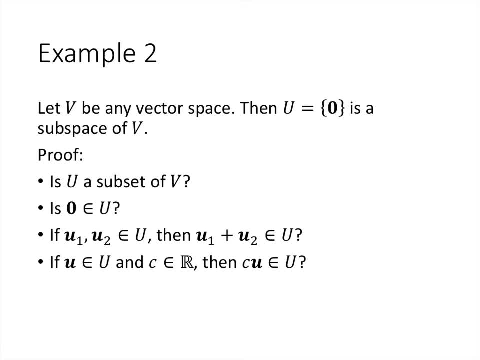 any vector space. then the set U that contains just a single vector, just the zero vector. that turns out to also be a subspace, a very small subspace. So, first of all, is it a subset? Sure, it only has one element in it, and that element is an. 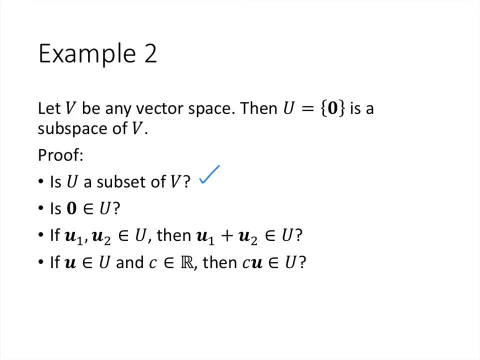 element of capital V. so U is a subspace. Is the zero vector in capital U? Well sure, it's the only element of capital U. so that's true For this third bullet, if we take two elements of capital U and add. 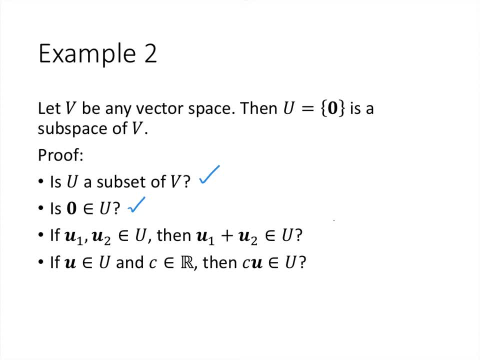 them together is the result in capital U. Well, the only thing we can take from capital U is the zero vector. so the only thing we have to check is that when we add the zero vector plus the zero vector, well there we get the zero vector, and 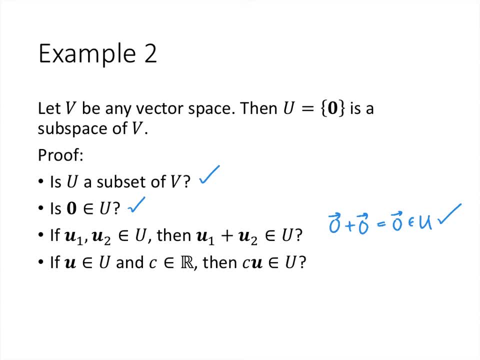 that is in capital U. And then, finally, if we take something out of capital U, well, there's only something, there's only one thing we can take out of capital U. and if we multiply it by a scalar, well, multiplying the zero vector by any, 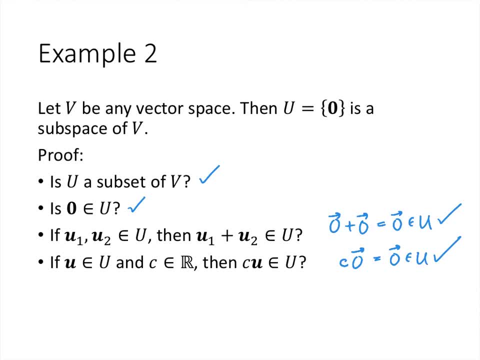 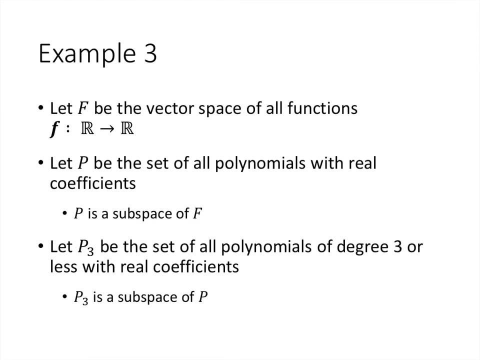 scalar just gives you the zero vector that's in capital U, so that checks out. Sometimes we call this the trivial subspace, because there's only one thing in there and it's just the zero vector. Look at another example. So earlier we 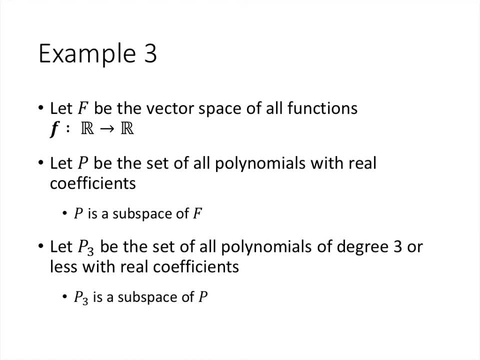 talked about the vector space of all functions, from the real numbers to the real numbers. so if we look inside that set of functions and find the set of all polynomials, well, polynomials are functions, so that's a subset and it's also a subspace. If we add two polynomials, we're going to get another. 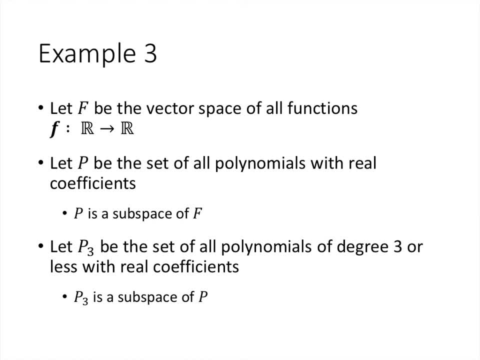 polynomial. if we multiply a polynomial by a scalar, we get another polynomial and the zero function is a polynomial. f of x equals 0, that is a trivial polynomial. And then, inside of the set of all polynomials, if we look at the 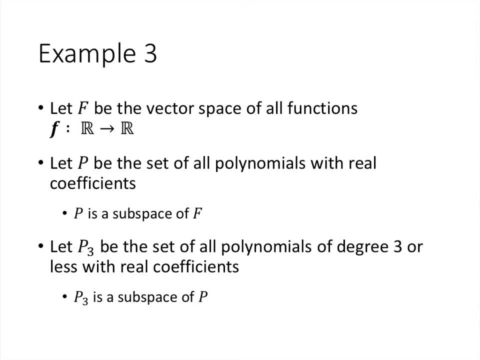 set of all polynomials of degree 3 or less, then that's also a subspace, because if we add two of those polynomials with degree 3 or less, we get another polynomial with degree 3 or less, And if we multiply a 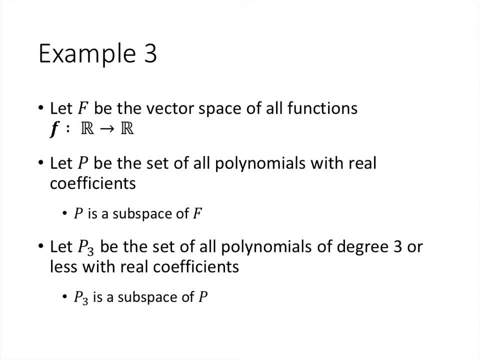 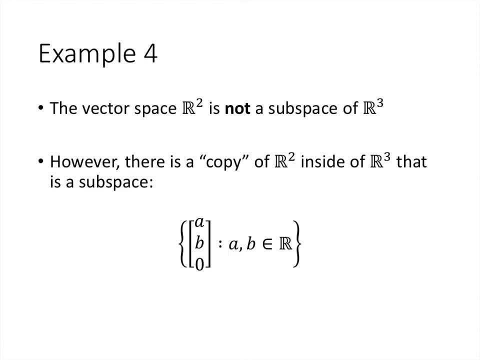 polynomial with degree 3 or less by a scalar, we get another polynomial with degree 3 or less And again the zero polynomial does have degree 3 or less. Let's look at a couple non-examples. So the vector space R2 is not a subspace of R3,. 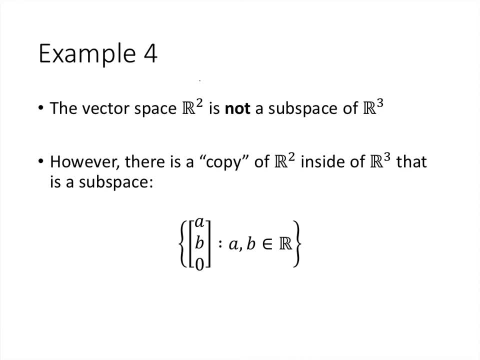 because it's not even a subset of R3.. The elements of R2 have two entries and the elements of R3 have three entries, So R2 is not even a subset of R3, so it can't be a subspace. 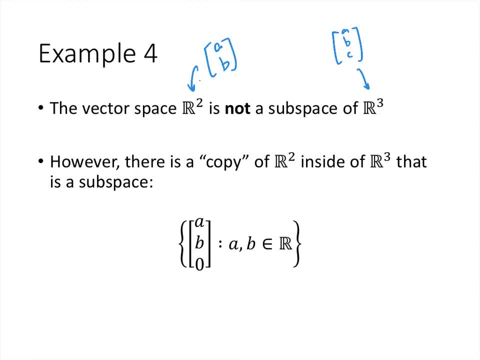 Now there is a copy of R2 inside of R3, so we can think of this as being the xy plane in our three-dimensional space, And so this is a subspace, this set of vectors that look like a b 0, and we can prove that this set is a subspace using the same method that we did before. 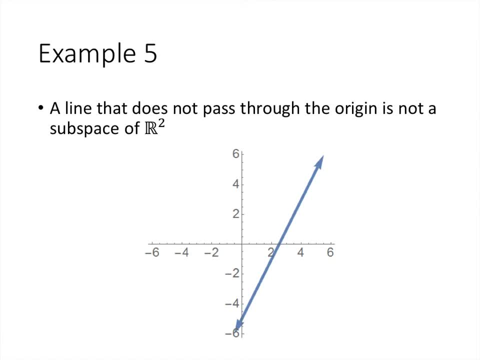 Another non-example is that a line that does not pass through the origin is not a subspace of R2.. So a couple reasons why: First of all, since it doesn't pass through the origin, it doesn't contain the zero vector And secondly, it's not going to be closed. under addition, If I take this vector in my line and 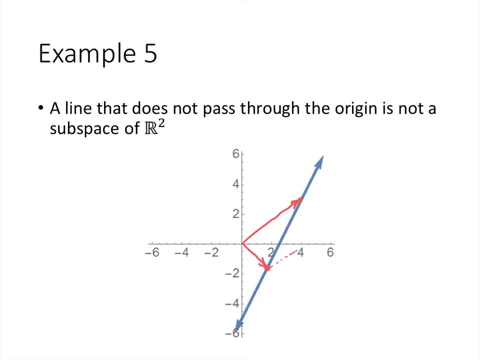 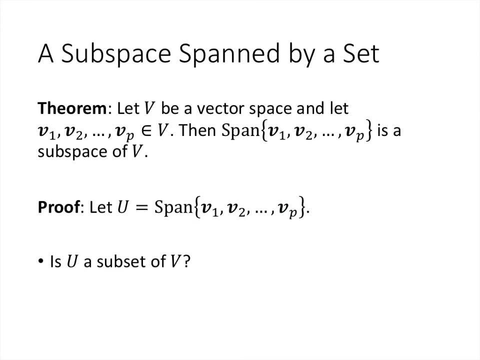 add it to this vector in my line, using my parallelogram rule for adding vectors, the sum of those two vectors is going to look something like this, and that's not on my line Now. an important example of subspace is the subspace spanned by a set. So this is the general 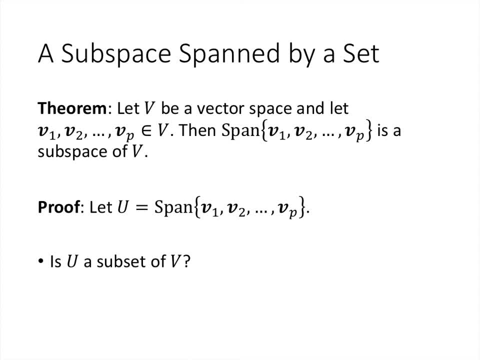 theorem true about any vector space, and it says that if you take some number of vectors in your space- v1 through vp- and look at the span of those vectors, then that span is a subspace. So we're going to prove it the same way that we proved it before. We've got four things to prove. 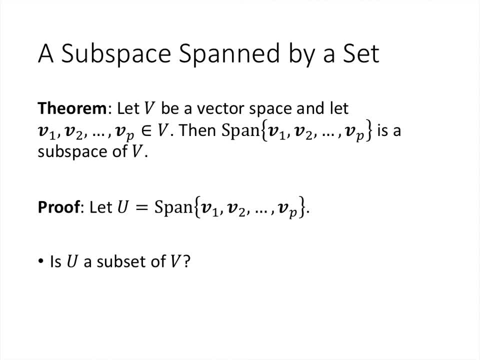 We've got to prove that u is a subset, we've got to prove that u contains the zero vector, and then we've got to prove that u is closed under the two vector spaces. So, first of all, is u a subset of v? Well, every element of u. 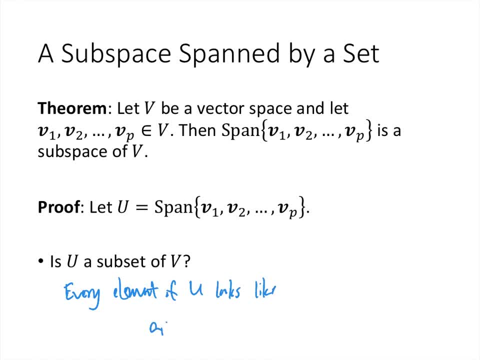 has the form a1, v1 plus a2, v2 plus plus, plus plus ap, vp. and since v is closed, under the vector space operations- scalar multiplication and vector space- that's certainly an element of capital V and that shows that u is a subset of v. 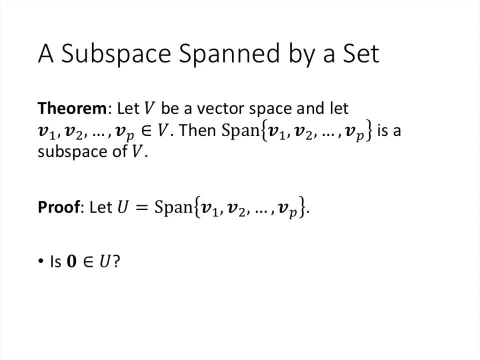 Is the zero vector in capital U. Well, again, the answer is yes because, remember, u is the set of all possible linear combinations of those v vectors. and so to get the zero vector, all we're going to do is take the linear combination where we use the coefficients of all zeros. 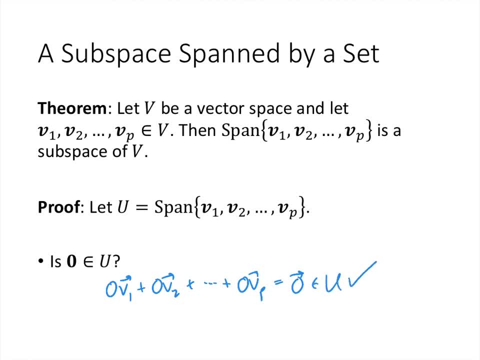 So that's going to work out to be the zero vector and that will be in capital U. So the set of all possible linear combinations of all zeros is the set u closed under addition. Well, now what we have to do is if we take two of these linear combinations of the little v vectors, 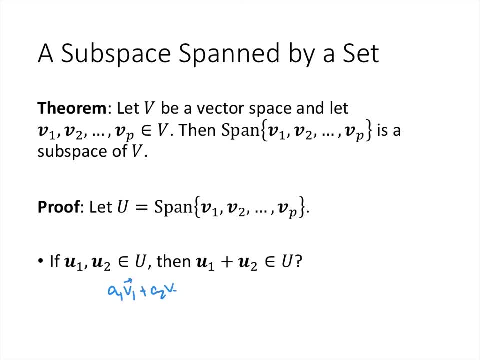 and add them together, do we get another linear combination. So in other words, if we let a1 v1 plus a2, v2 and so on, and if we add that to some other linear combination- b1 v1 plus b2 v2,. 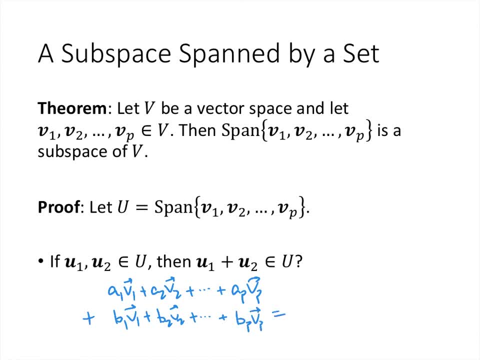 we get a set u closed under addition. If we add those together then that is going to be a linear combination. So that's a1 plus b1 times v1,, a2 plus b2 times v2, plus, plus, plus all the way up through ap. 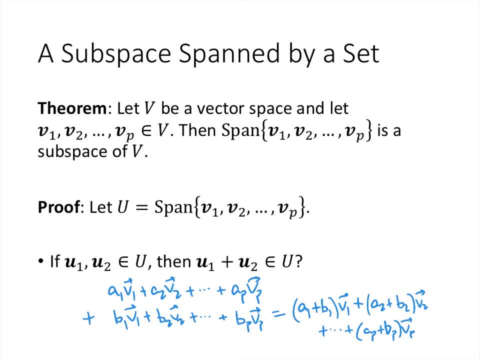 plus bp times vp, And since that's a linear combination of the v vectors, that's in capital U. Finally, if we take an element of capital U and multiply it by a scalar, do we get another element of capital U? So, in other words, if we take 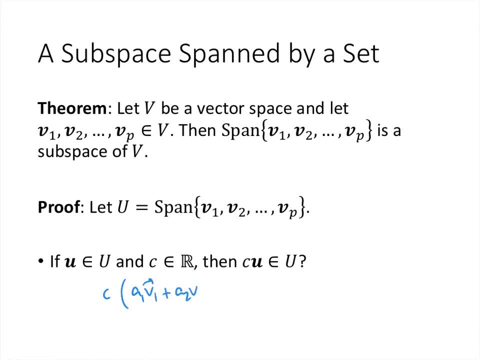 one of these linear combinations- a1, v1 plus a2, v2 plus plus, plus plus ap, vp, and multiply it by a scalar c, well, what we get is c times a1, v1 plus c times a2, v2 plus plus, plus plus c times ap, vp.